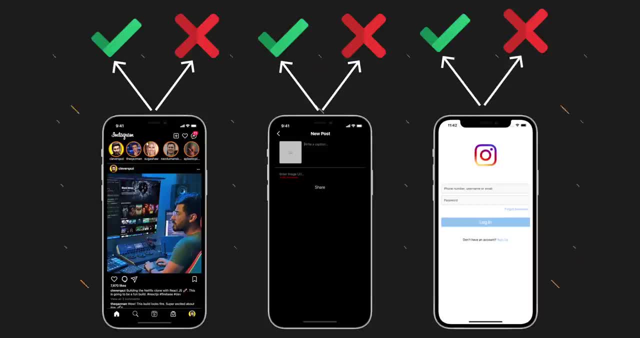 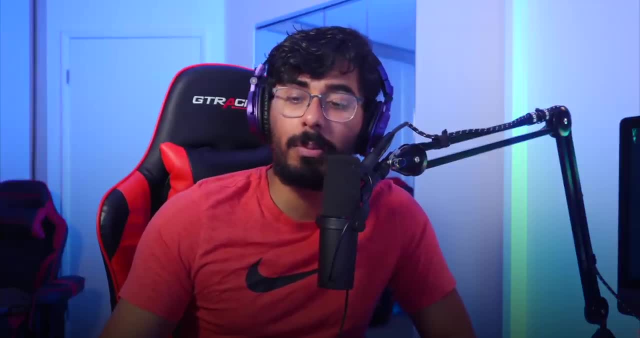 going to have to manually do it on every single screen. So wherever we wanted to essentially show stuff, we would need this conditional rendering. And we're like man. this seems like it's not following the dry principle, right Like don't repeat yourselves. Don't repeat yourselves. 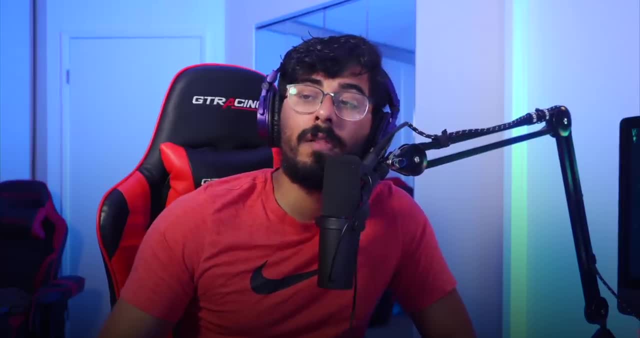 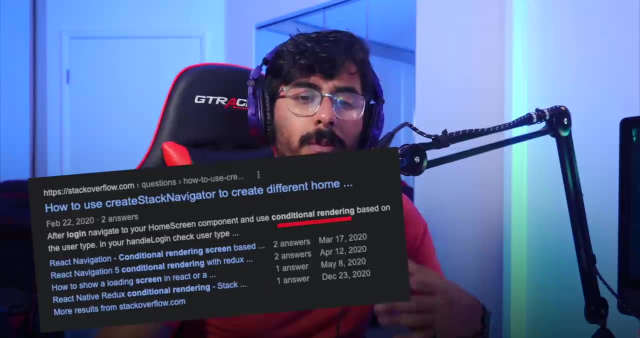 Don't repeat yourselves. So I thought how could we make this authentication workflow better? So I started scouring the internet and I wasn't able to really find super helpful stuff. A lot of people were just doing conditional rendering on each of the screens and then nobody was really showing. 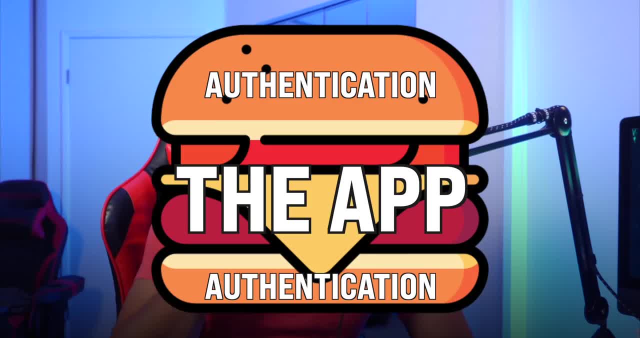 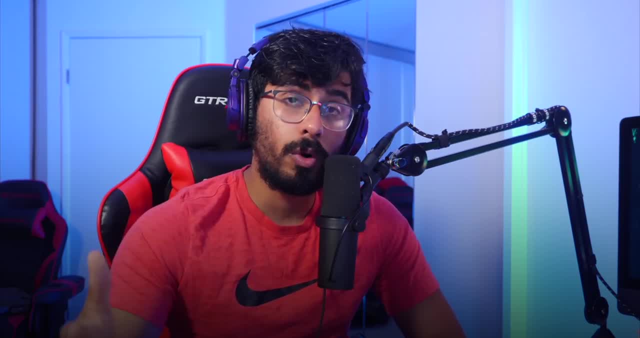 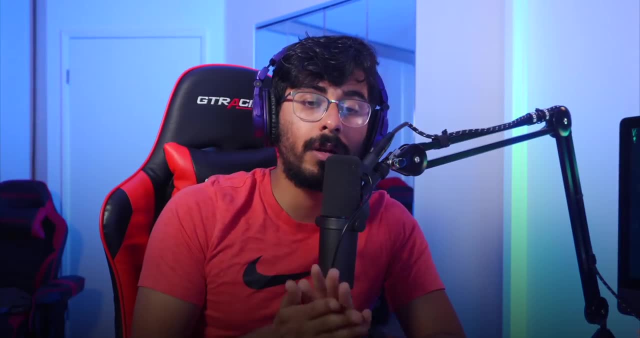 how to wrap the entire app inside of authentication. And then I came across this amazing article and he was talking about how you can implement the authentication workflow where, essentially at the global level, where you put your root navigation in React Native, at that point you want to wrap it right And you want to add a Firebase authentication listener to it. 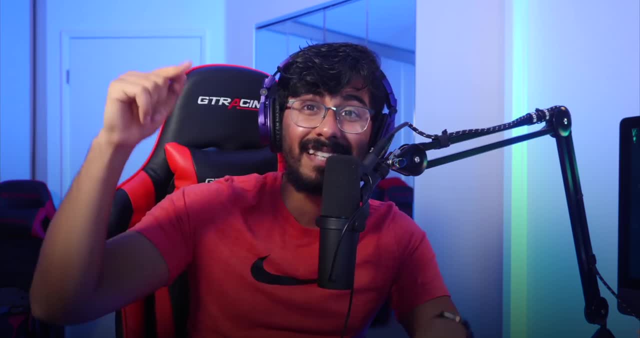 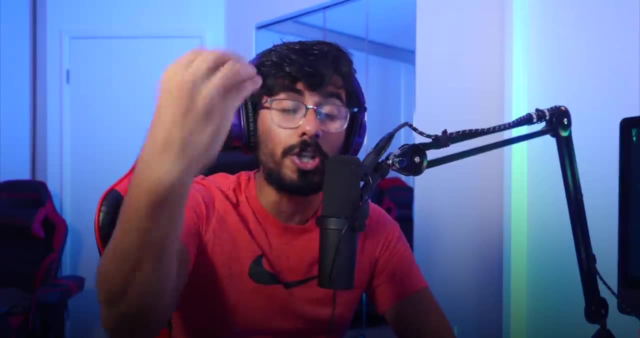 at the global level. And then what he was doing is he was building a sign-in stack and then he was building, essentially, a signed-out stack And I was like yo, this is genius. So we took that idea and we're like that is such a clean way of doing it Essentially. 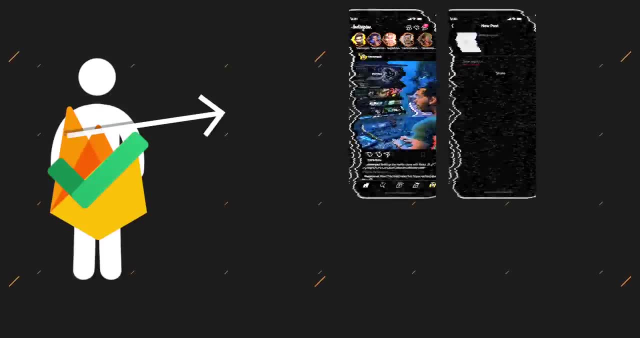 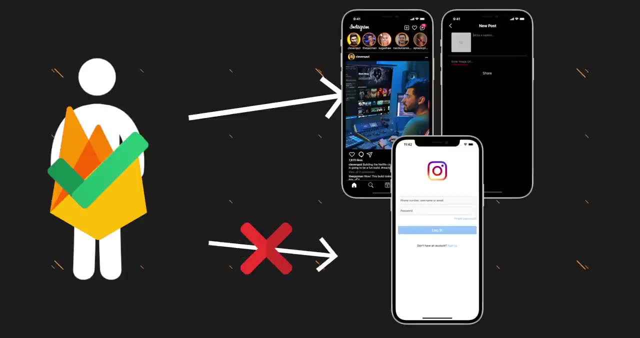 it's going to be so sick because, if you're logged in, you will be given the sign-in stack at the global level, meaning that your stack won't even contain the login and register screen, So it's impossible for you to have access to them. Just to describe to you what sign-in stack is right: 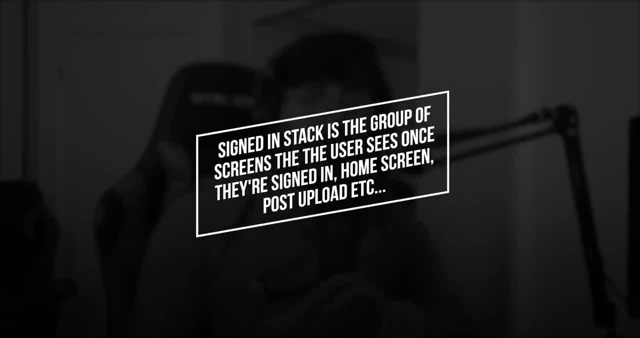 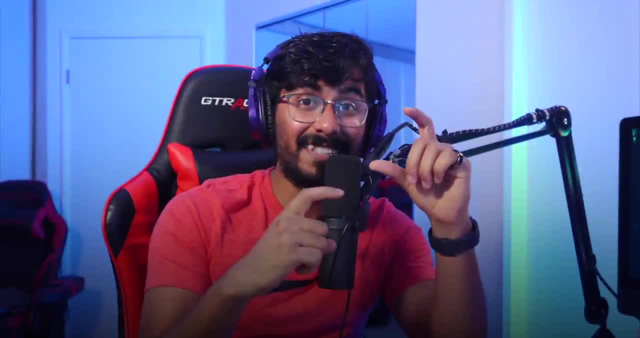 Sign-in stack has access to all the screens the users should have when they're signed in. The signed-out stack has two screens: the login screen and the sign-in stack. So if you're registered screen, so you create these two stacks, Because the other way of doing the 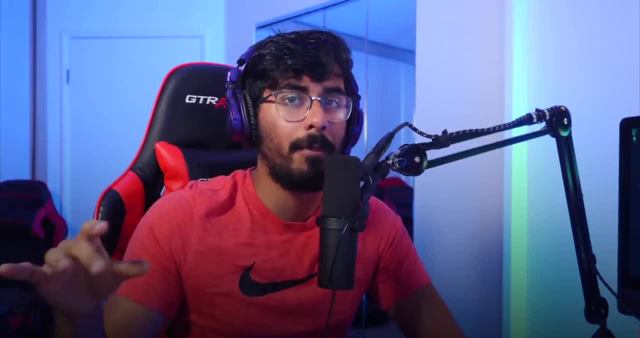 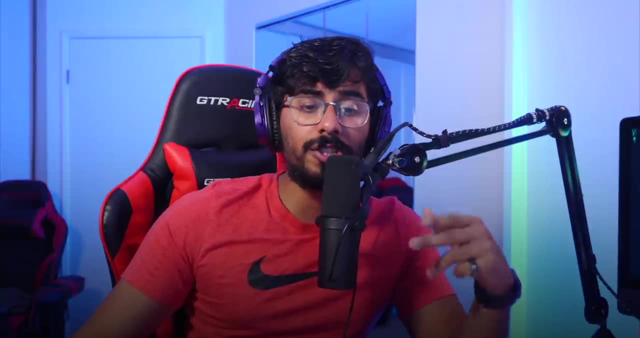 conditional rendering. there's some security issues too, where some weird bugs can happen. right, But at this level they won't even have access in their screen stack to these screens at all, And I thought this was such a genius way of doing it. Another benefit to this was I was running 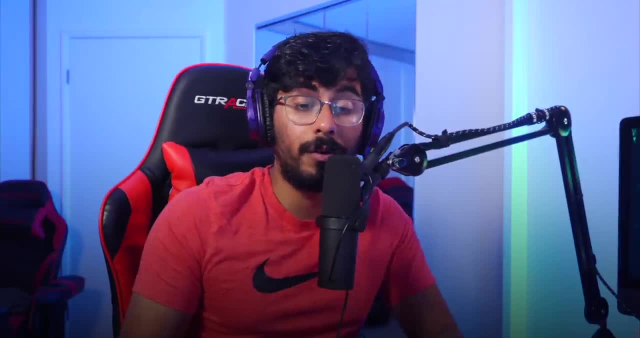 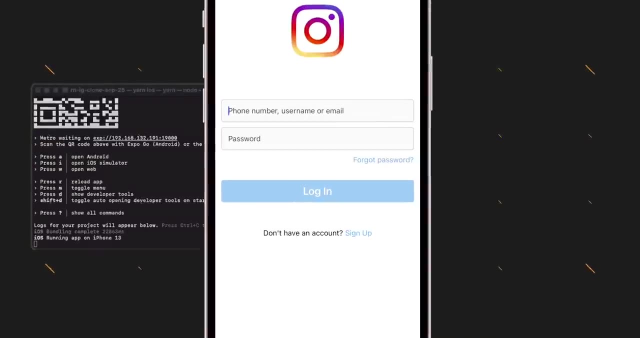 into this other problem right. The older way of doing it, how we were doing it earlier, If you log in, the problem was that if you refresh your app, it would start you back from the login screen right, And so the other solutions would be. 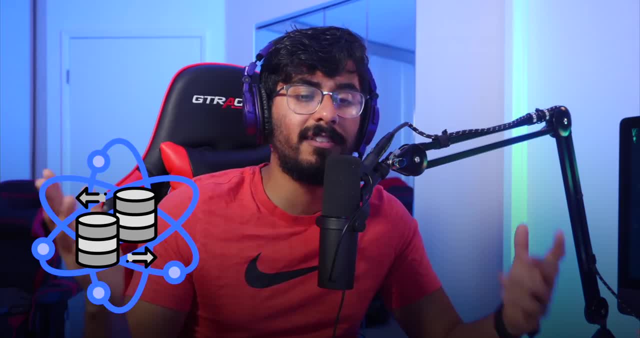 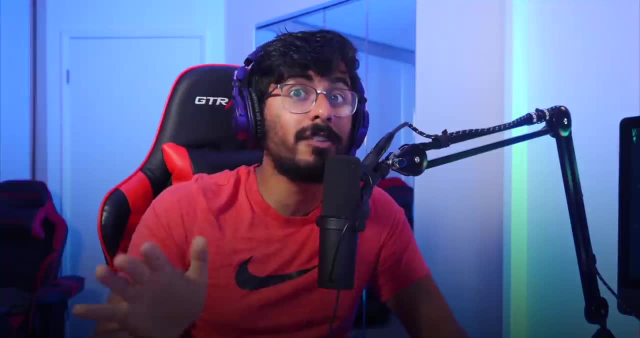 oh, Kazi, just use local storage. Oh yeah, React Native just has async storage. It just does this, just does that. It's not necessary If you do it the right way. the right way is so freaking clean that none of this crap is necessary at all. Firebase has this really nice listener. 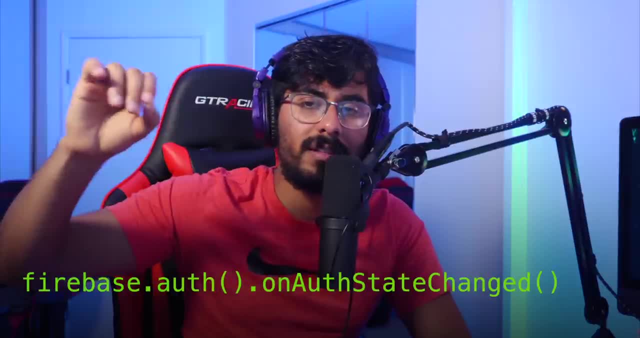 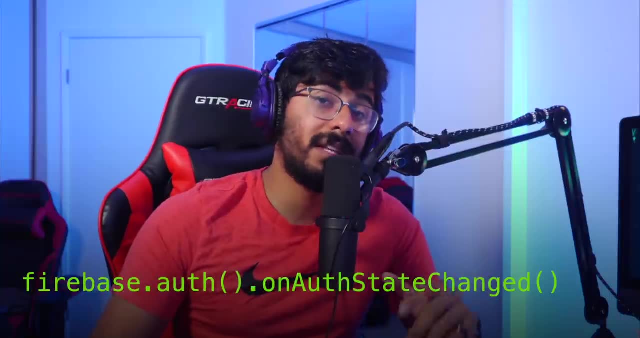 You know, you basically do like Firebaseauth and then you want to do onAuthStateChanged And this is a listener that Firebase gives you And it's detecting any time the authentication changes, meaning any time the user either logs in or signs out, and it's listening. 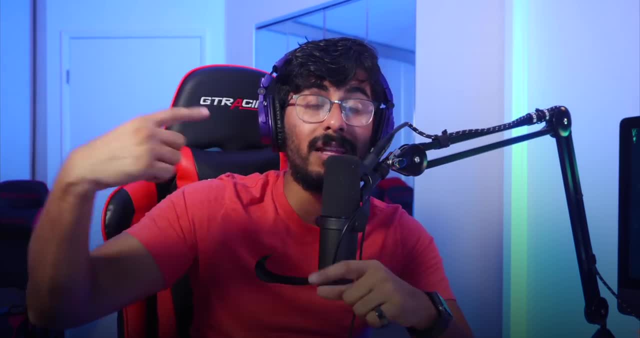 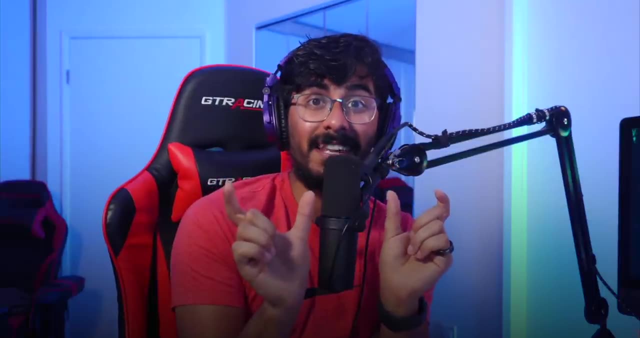 So if we wrap the entire app at a global level in this listener, it'll always be listening, no matter what screen they're on. And then here's what we do: If user is logged in, give me the signed in stack. Otherwise, give me the signed out stack. It is so freaking beautiful. It was so fun. 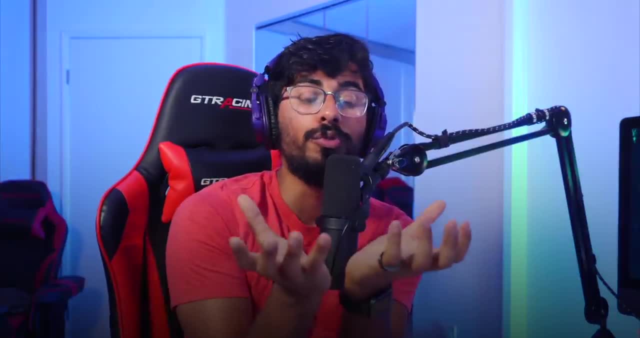 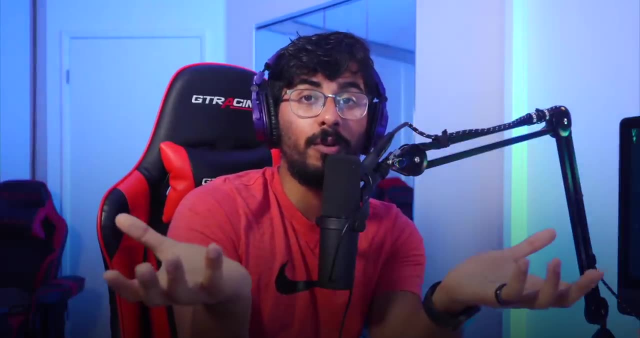 writing this if and then statement because it's literally like you created two universes, like your signed in stack and your signed out stack. You create these whole two worlds And, depending on if this or that, you put them in a whole new world. right, If the user signed in, put them in. 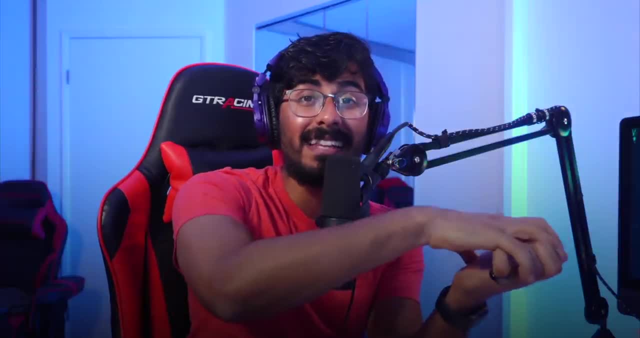 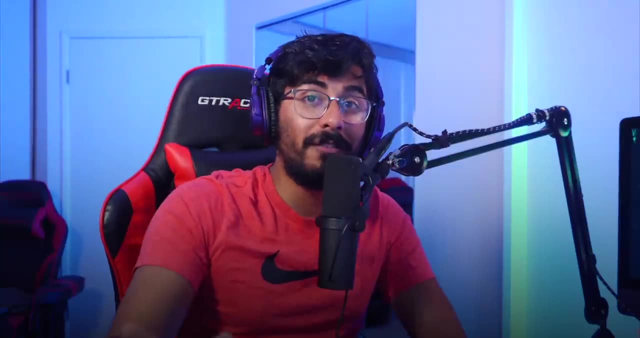 and that's all they have access to. Or, if they're signed out, put them in the signed out stack world And that's a whole universe in itself that they're in, and then they can't get out of it right So secure. And then here are the other benefits of it, And this is what I love the most. So usually, 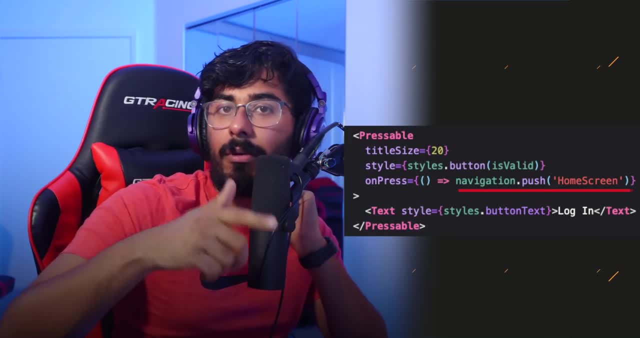 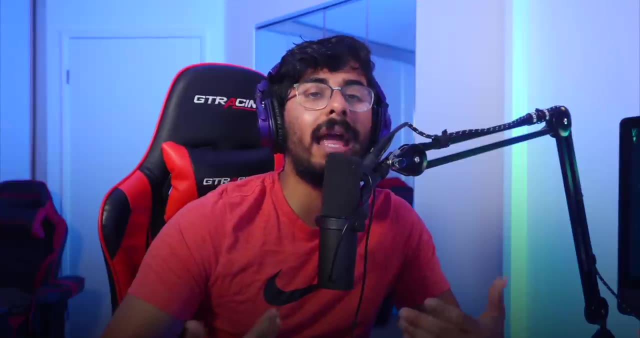 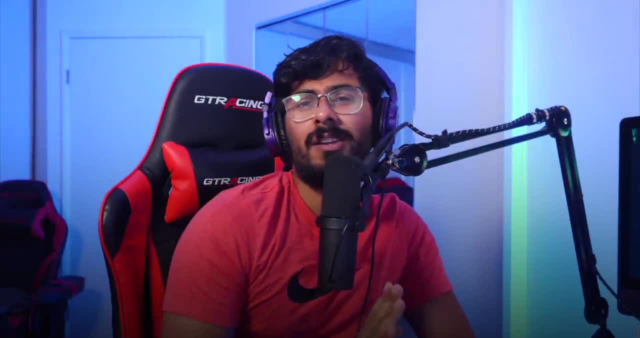 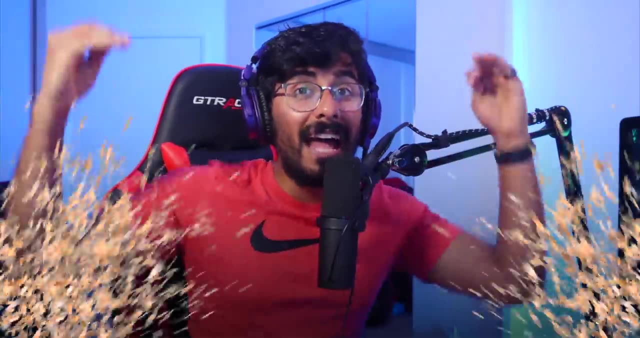 It took you back to the login, Like how would that make sense? You just logged in, It shouldn't even let you go back to it. And so, with this new way of doing it, you don't even have access to the login or register screen anymore. So as soon as you log in, boom, now you're just in this whole. 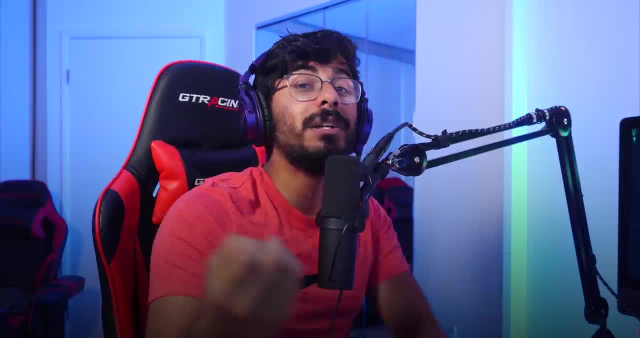 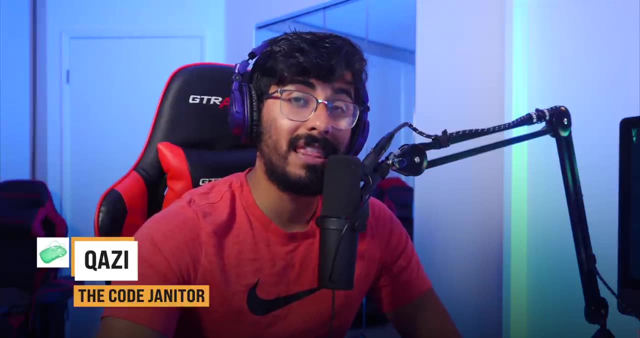 new world And if you try to swipe back, you can't. Experience is so much smoother. The security is so much smoother. Man, it is so freaking nice, But that was such a clean thing. I'm really excited about showing you guys this build when we drop it, So I'm going to show you guys how to do it. 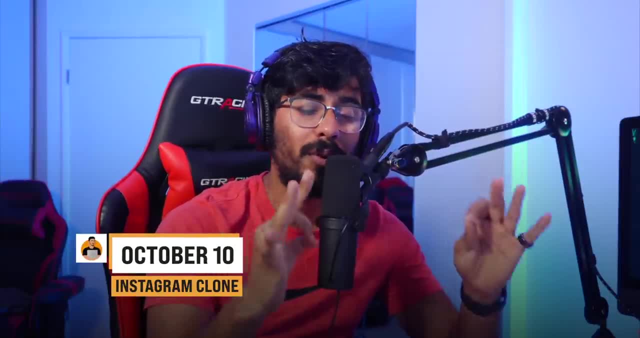 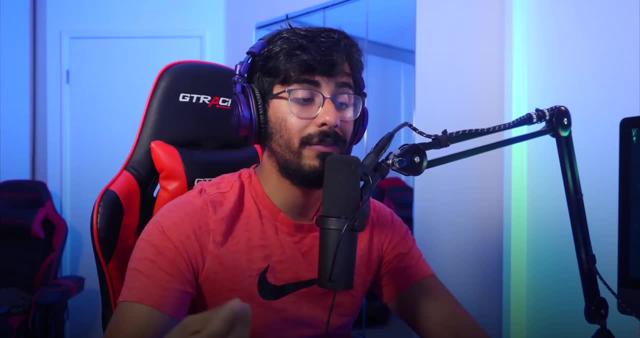 I think that for a lot of people, they'll have the super clean way of wrapping their entire up in this type of authentication And I really hope it provides a lot of you guys with a lot of value. So that's it, guys. Hope you enjoyed this video. Smash the like button. subscribe to this channel.